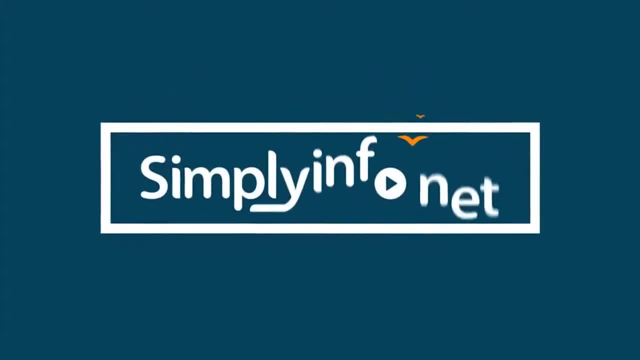 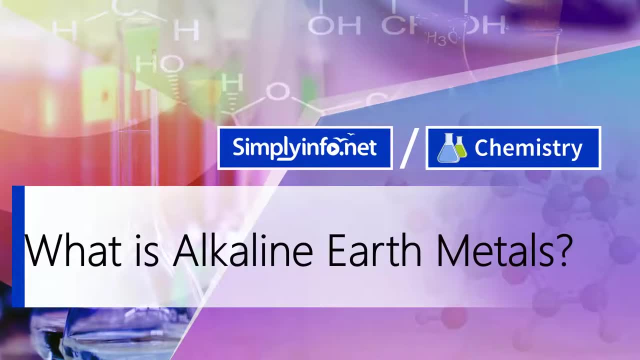 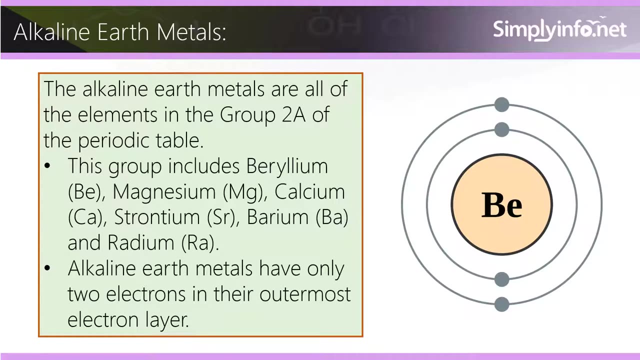 What is Alkaline Earth Metals? The Alkaline Earth Metals are all of the elements in the group 2A of the periodic table. This group includes Beryllium, Magnesium, Calcium, Strontium, Barium and Radium. Alkaline Earth Metals have only two electrons in their outermost. 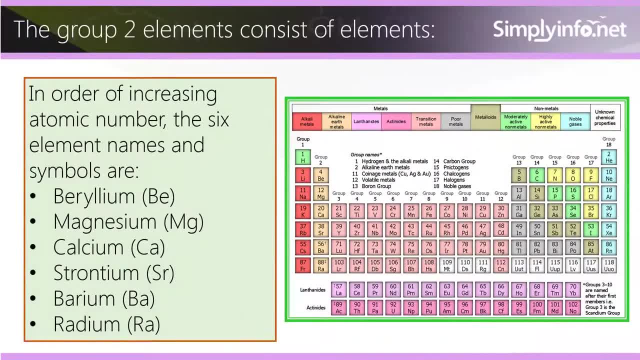 electron layer. The group 2 elements consist of elements In order of increasing atomic number. the six elements' names and symbols are: Beryllium, Beryllium and Beryllium, Magnesium, Calcium, Strontium, Barium, Radium. 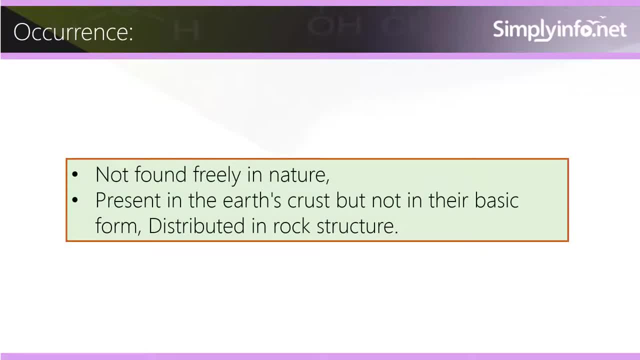 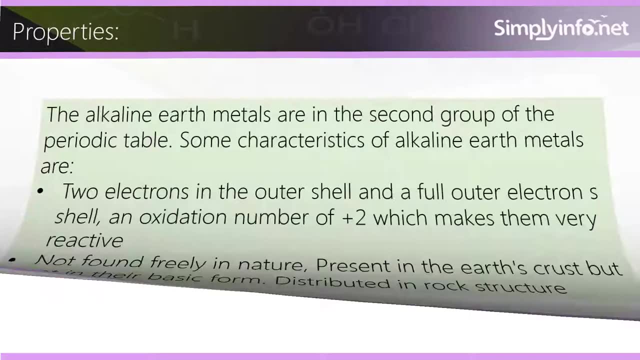 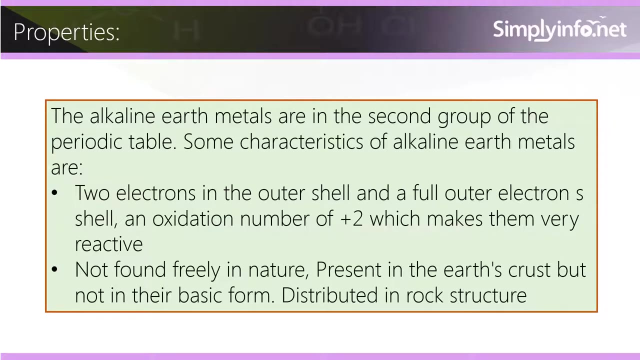 Occurrence Not found freely in nature, Present in the Earth's crust, but not in their basic form, Distributed in rock structure Properties. The Alkaline Earth Metals are in the second group of the periodic table. Some characteristics of Alkaline Earth Metals: 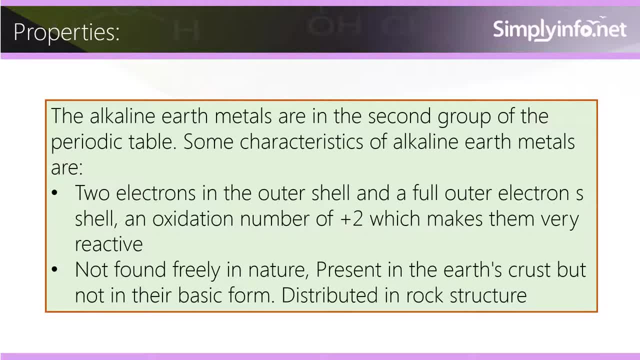 are- 2 electrons in the outer shell and a full electron shell, an oxidization number of plus 2, which makes them very reactive. Not found freely in nature, Present in the Earth's crust, but not in their basic form, Distributed in rock structure. 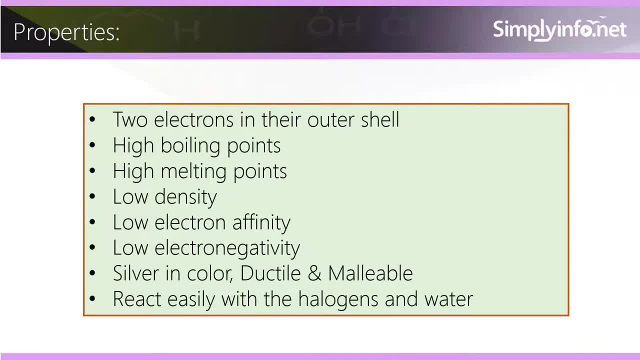 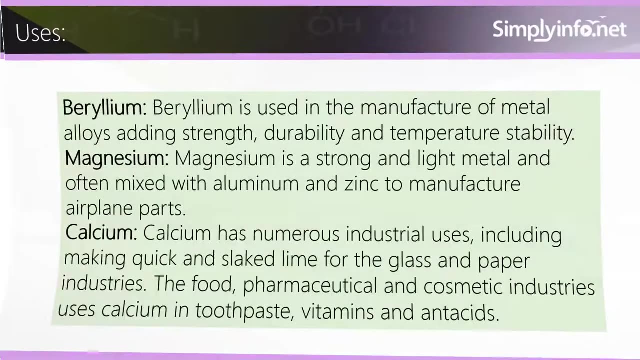 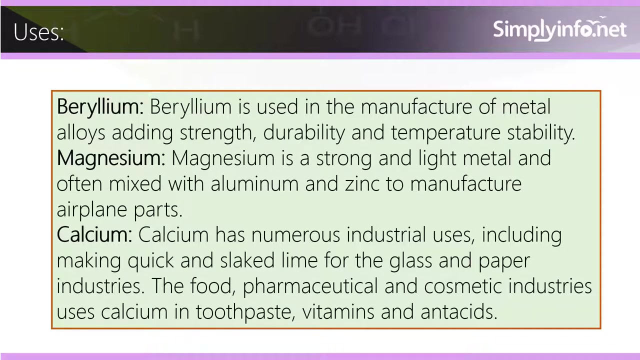 2 electrons in their outer shell. high boiling points, high melting points, low density, low electron affinity. Their use is 2. They 3. List Second Tip: 2. Best nes Calcium has numerous industrial uses, including making quick and slaked lime for the glass.